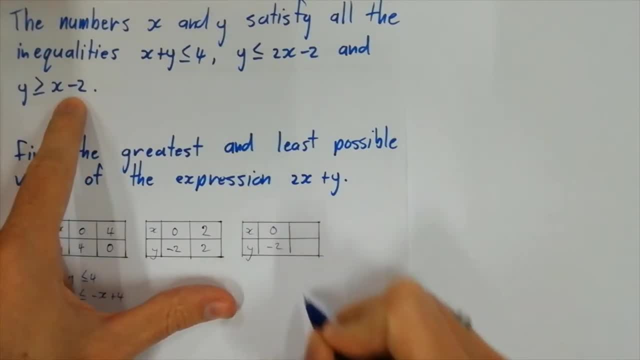 So if x is 0, y is minus 2.. If x is 2, y will be 0.. So already we have our three formula out here, We have our coordinates for them as well, And we can go ahead and plot the graph, And that's exactly what I want you to do now. 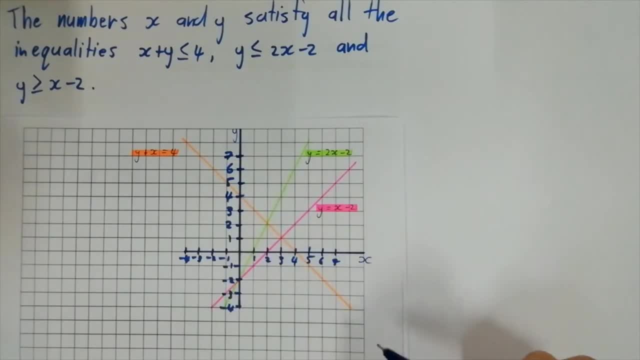 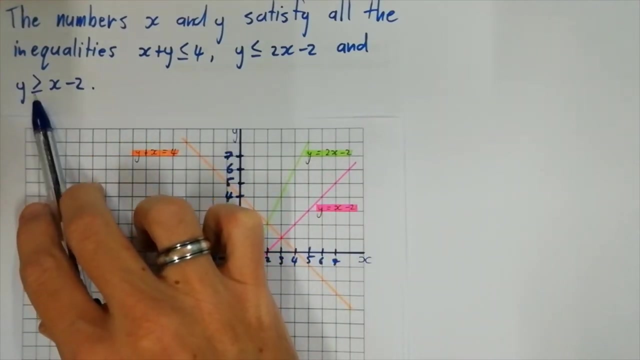 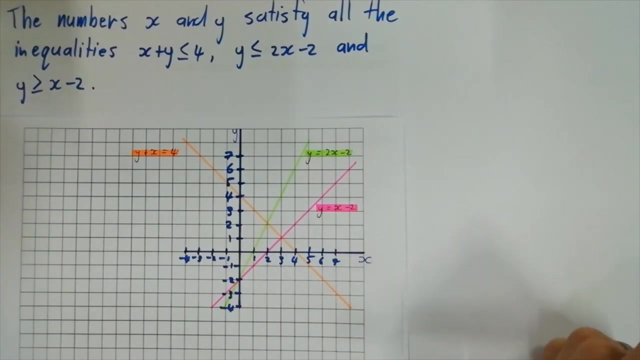 You should have a graph that looks something like this: We have some straight lines here. I know that these are all solid lines and you've made them so because they're all possibility, possibly an equal to, which is fine. But once you have this, we need to get on to the second part of the problem. 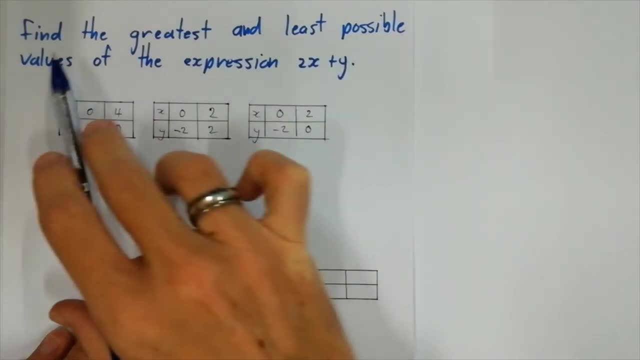 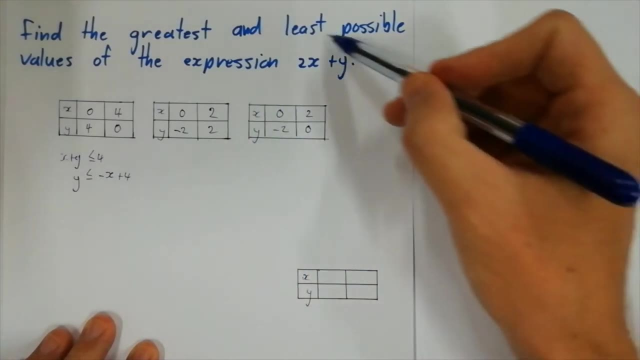 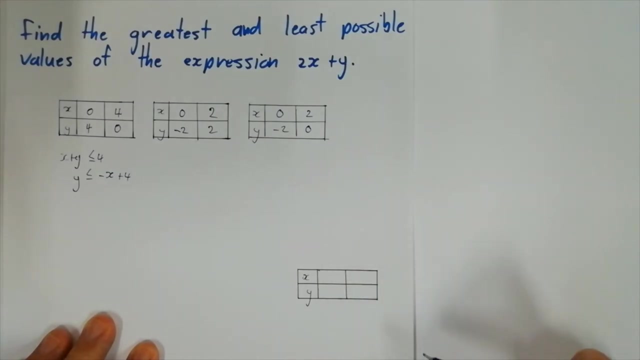 Find the greatest and least possible values of the expression 2X plus y. So the first thing we need to do for this is we need to get a line. We're going to use a formula over here. We're going to say: to negative 2x. if we're working with this, we can say: if X is 0, why would be? 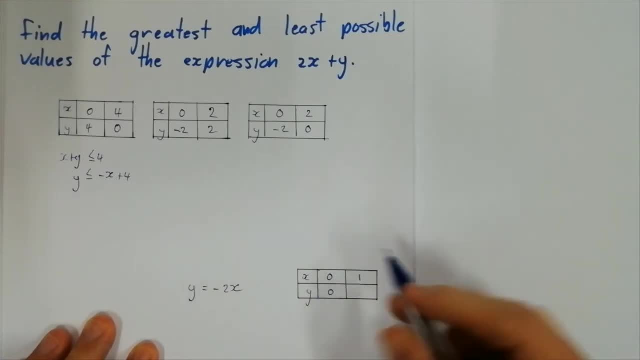 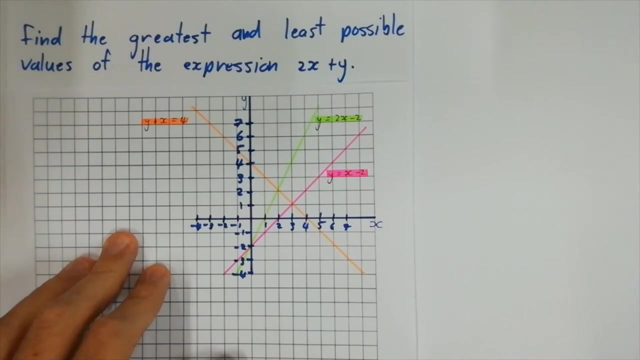 0 if X is 1. 1 times negative, 2 would give us negative 2, and now we can try and work out at what point we would find the greatest and least possible values of the expression. so let's get our graph ready. all right, we have two coordinates. 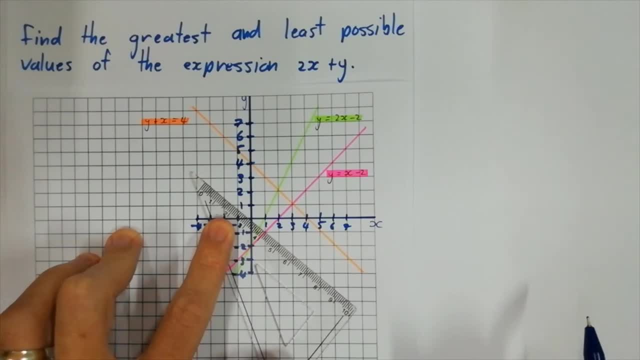 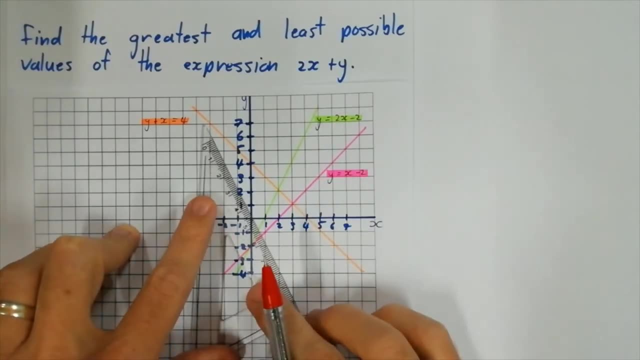 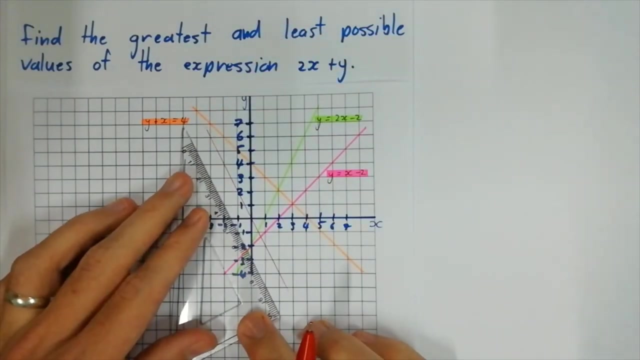 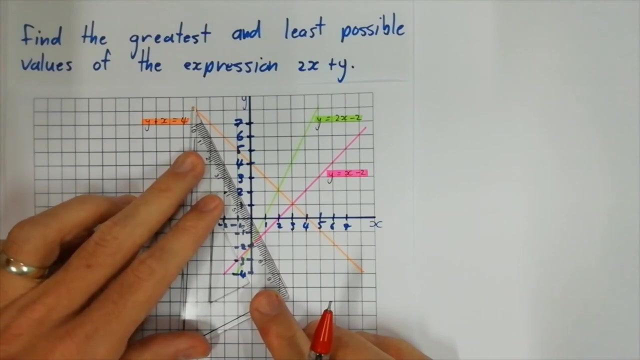 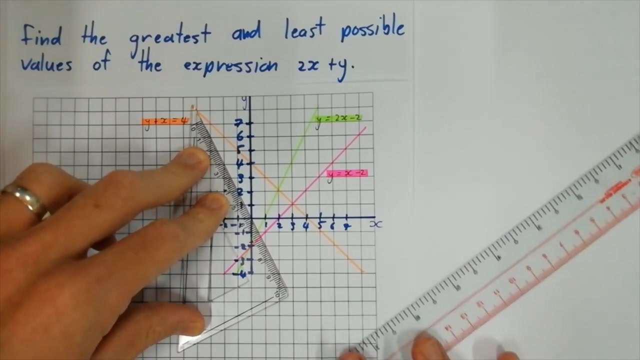 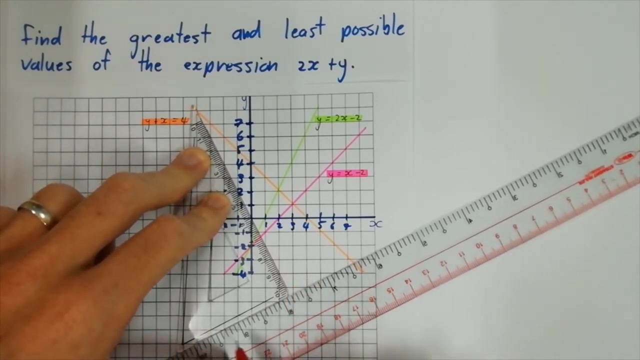 0, 0 and 1 minus 2, so our line will be formed somewhere along here, somewhere along here. so what you're going to do is you're going to place your set square on that line. take a ruler and place the ruler against the foot of the set square, so they're sitting against each other. 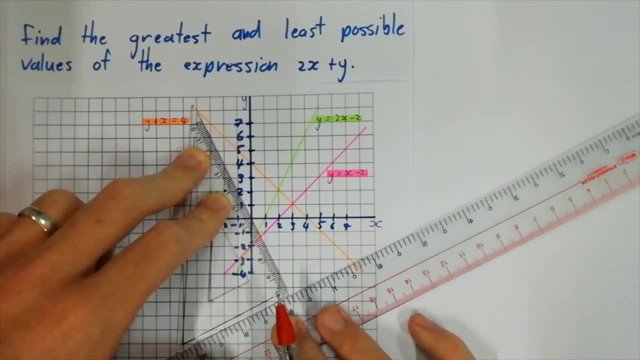 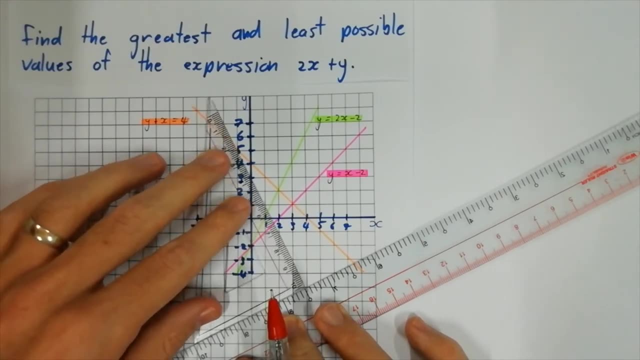 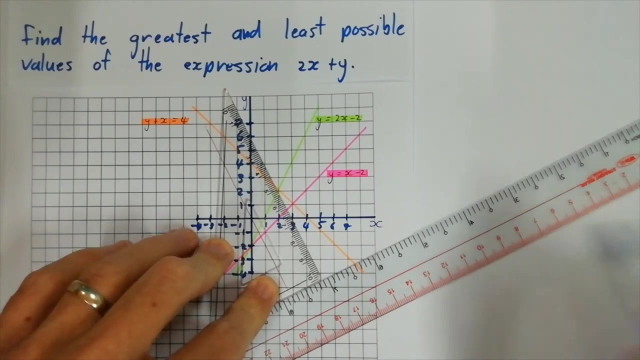 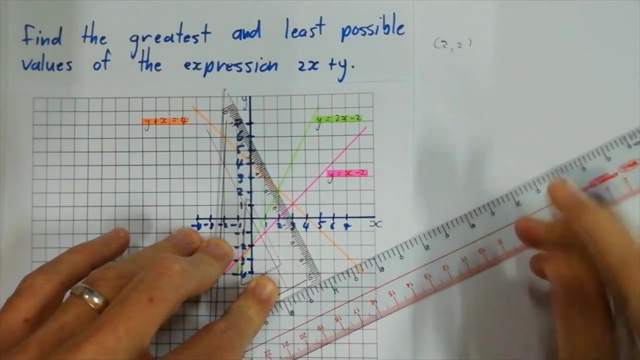 so they're sitting against each other. so they're sitting against each other. then we're going to slide the set square at the same line. using the same line, we're going to slide it up until we hit a point, and the point that we hit here is the point 2, 2. 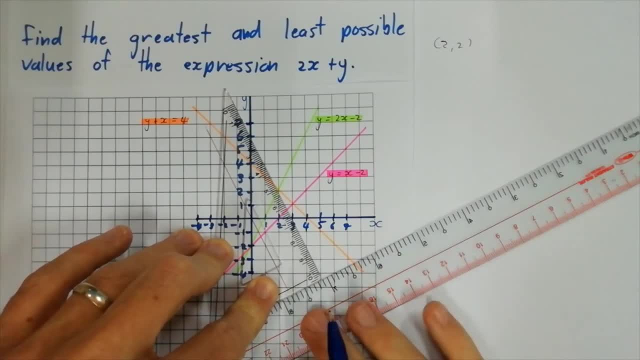 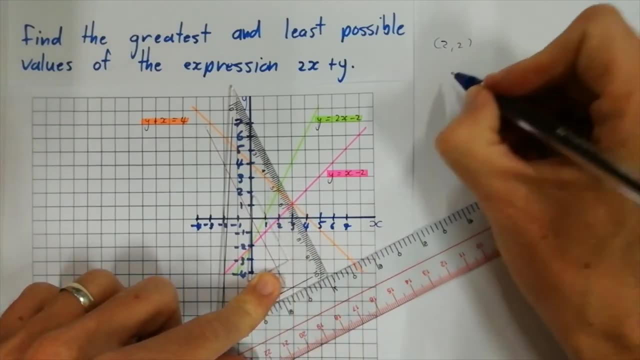 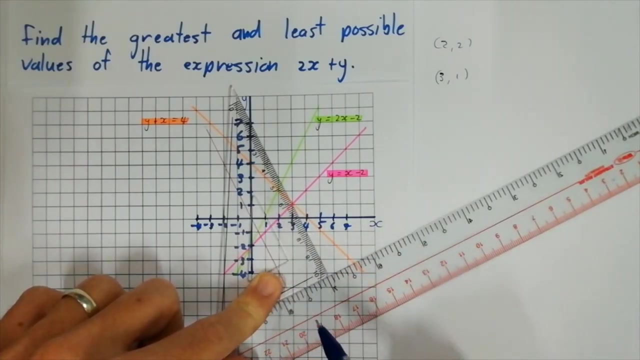 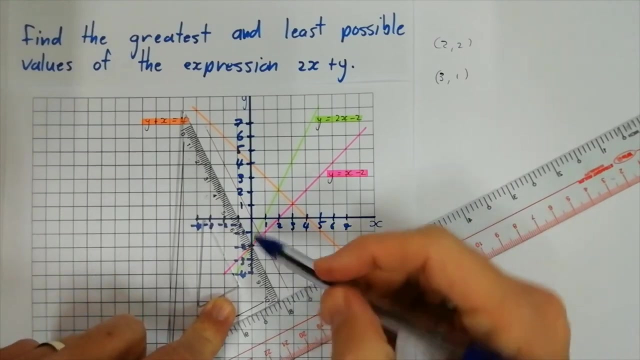 then we hit another point in this triangle and at this point we have 3: 1. x-axis is 3, y-axis is 1. let's move it down. we have another point in this triangle and this is 0 minus 2. this could be any shape, if it's a square, any sort of quadrilateral, you. 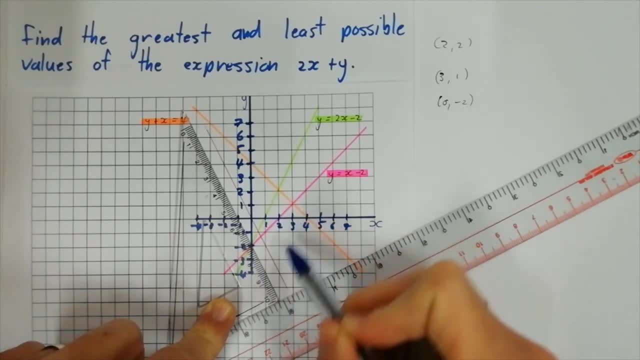 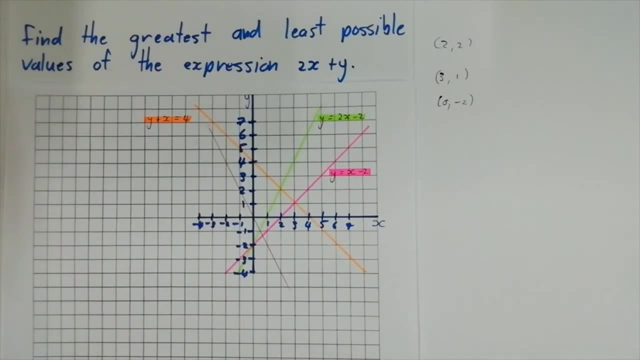 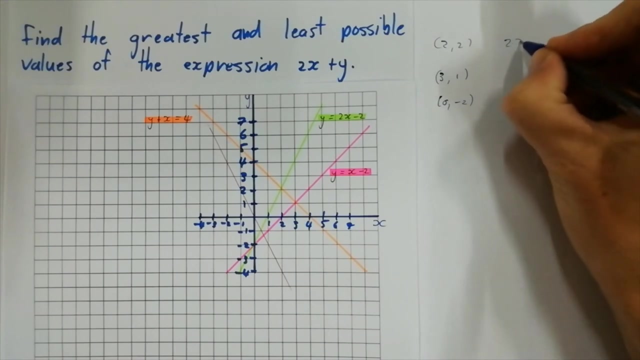 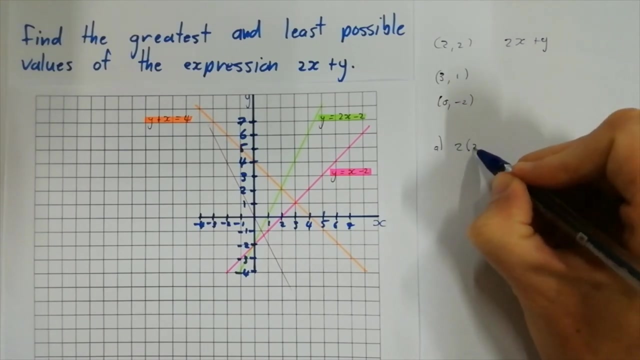 always go to the points. you always go to the points. now we can do away with these. we're done and we can start using our formula. our formula is 2x plus y. well, let's substitute the values in. so for our first point, we'll call this a. we will say 2, 2 plus. 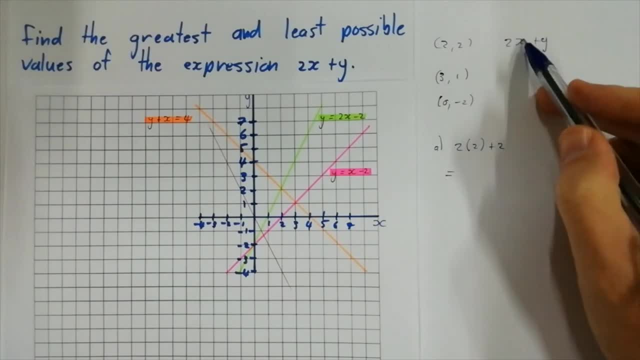 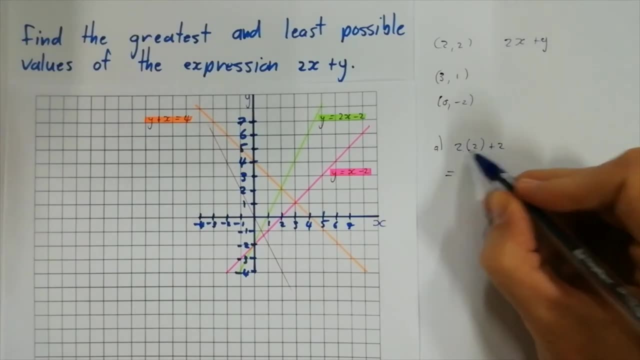 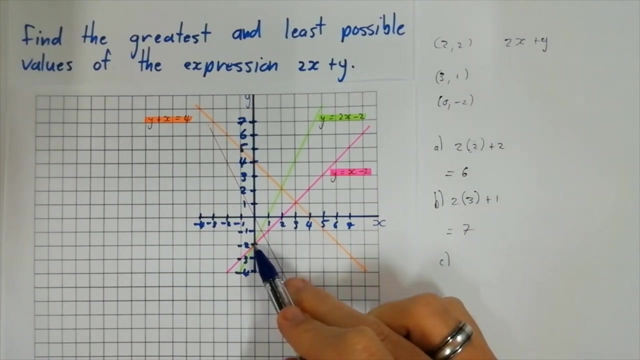 2, our y, our x value is 2. our y value is 2 as well, so that would give us 4 plus 2 is 6. next one: our x value is 3, so that is 2 times 3 plus 1, that would be 7. and the last point in our triangle at: 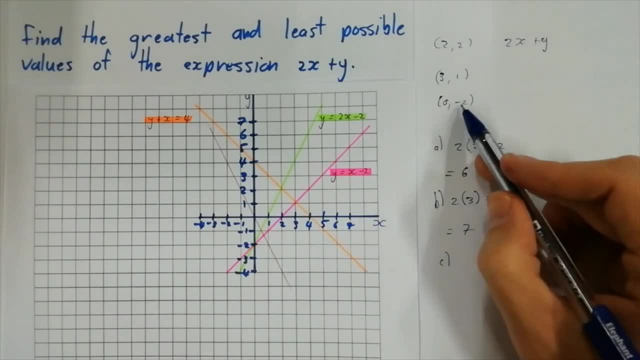 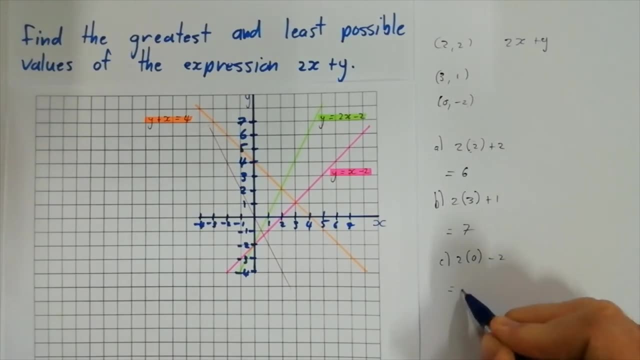 the bottom here would be 0 minus 2, so 2x would be 2 times 0 minus 2. this would give us negative 2. so what is the greatest possible value? well, the greatest possible value is 7. the least possible value, the least possible out of. 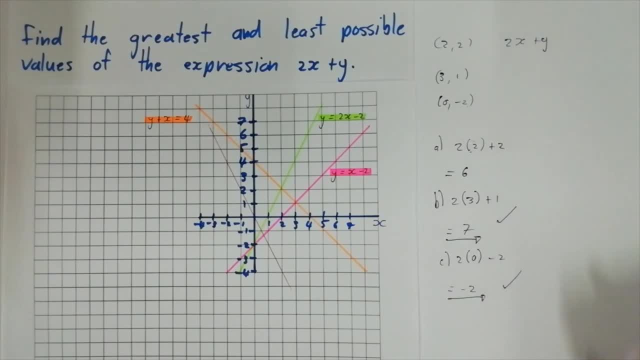 these three is negative 2. this is how we find the greatest and least possible values.